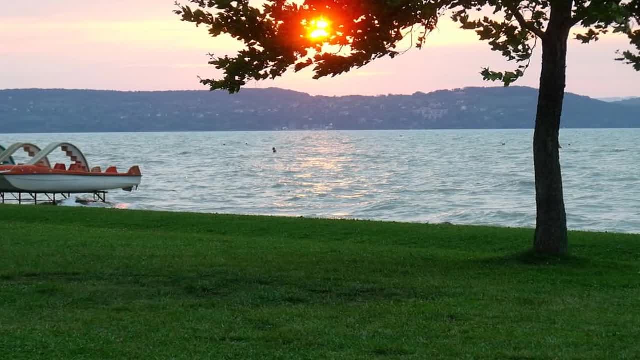 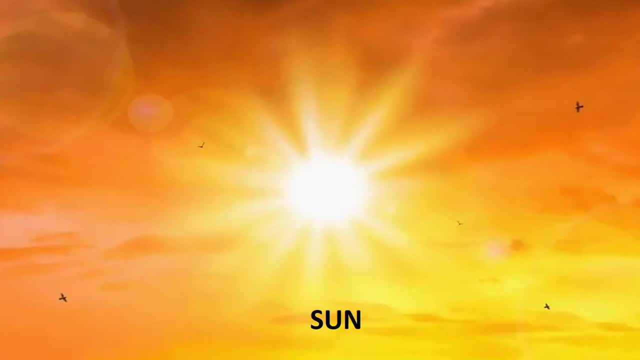 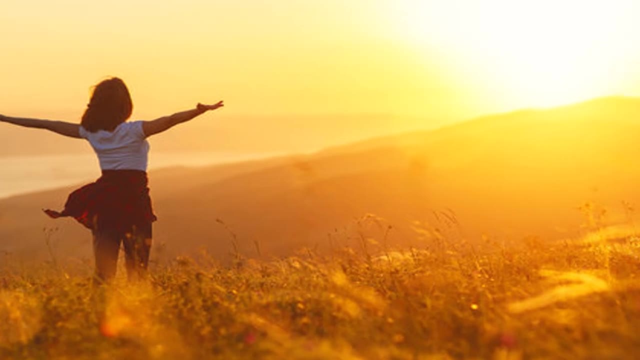 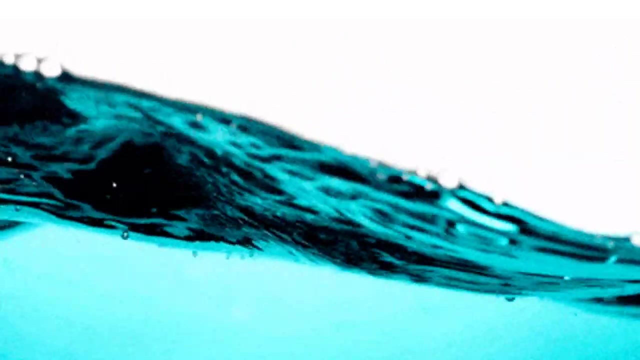 Renewable resources. A renewable resource is a natural resource that can be replaced easily within a human life span. Some examples are Sun. The light from the sun supports all the life on earth. It is also considered inexhaustible Water. Water is essential for all living things. It is constantly renewed by the water cycle. 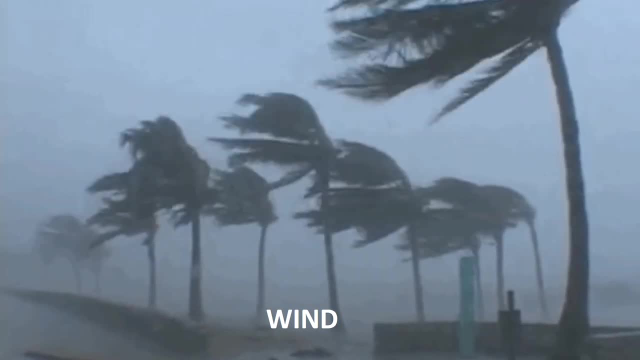 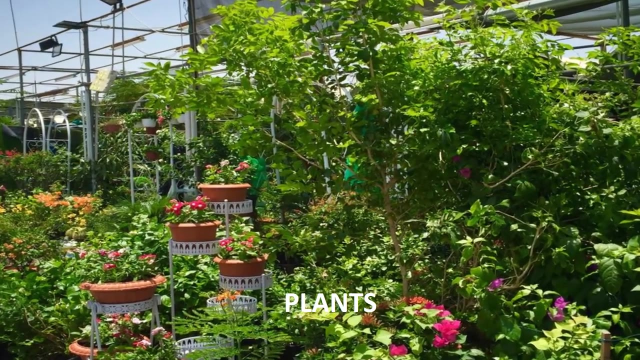 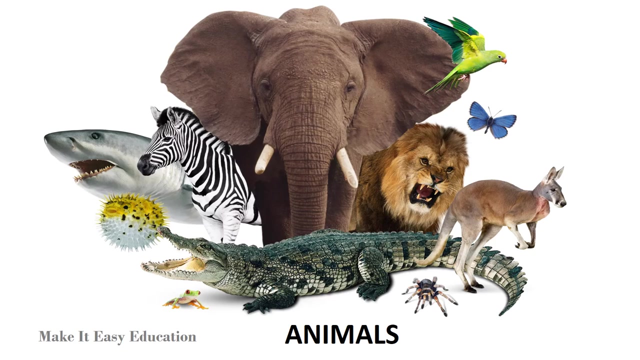 Wind. Wind is caused by the uneven heat of the earth. It is not only renewable but also inexhaustible Plants. Plants are renewable resources. If we cut down the plants, they can regrow from seeds and sprouts. Animals- Animals are renewable resources. Baby animals are born and grow. 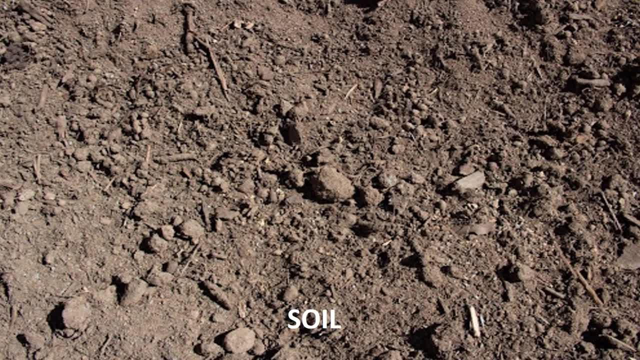 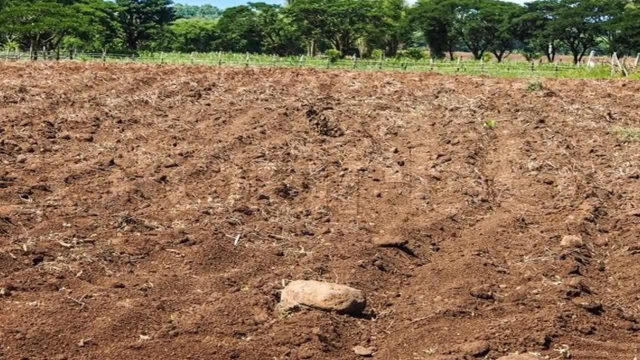 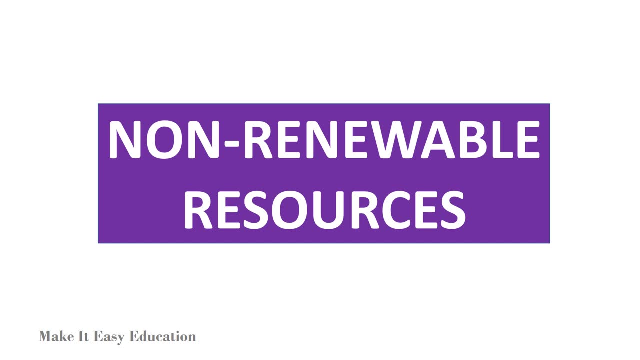 up. They replace older animals that die Soil. Soil is the thin layer of material covering the Earth's surface. It is made up of organic materials, air, water and living organisms. Non-renewable resources. Non-renewable resources are resources. 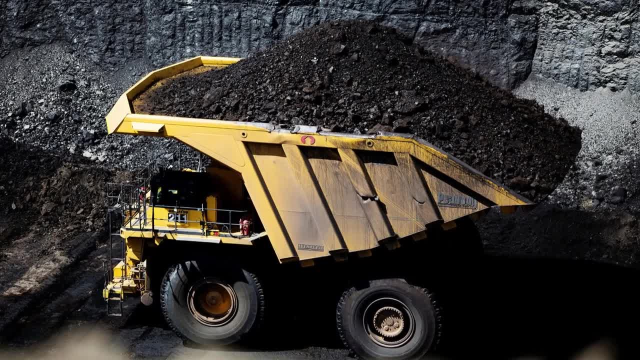 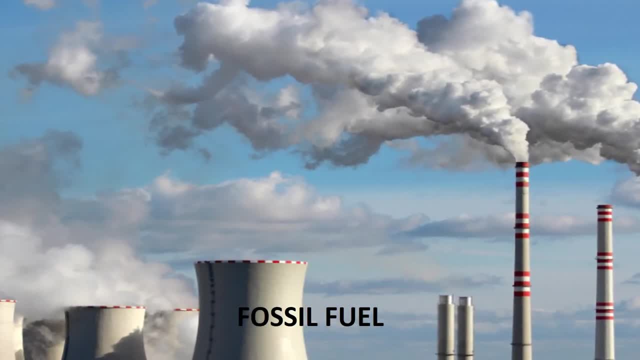 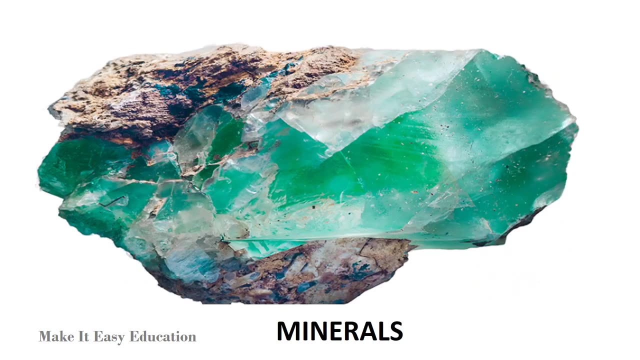 that can finish or be used up. It takes many year- that is more than a person's lifespan- to be replaced. Fossil fuels are non-renewable because they take thousands of years to form. The fossil fuels are mainly coal, oil and natural gas. Minerals are also non-renewable natural resources. It takes